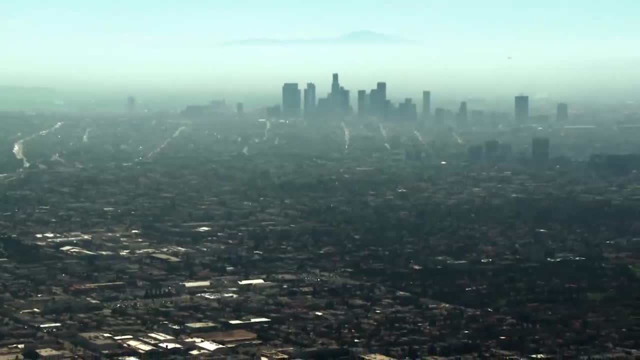 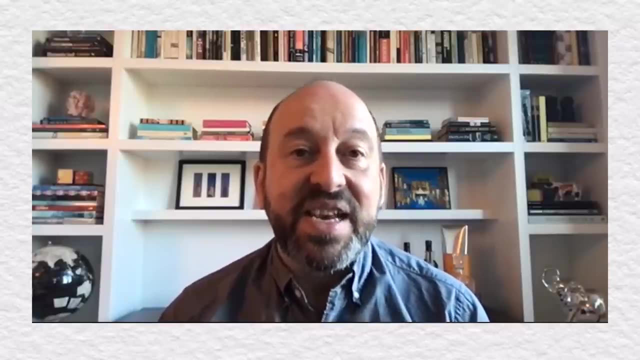 when humans started putting significant amounts of carbon dioxide in the atmosphere, But we'll get back to that later. There are millions of measurements over the last 140-odd years. We put those together. We're using data from literally tens of thousands of different stations. 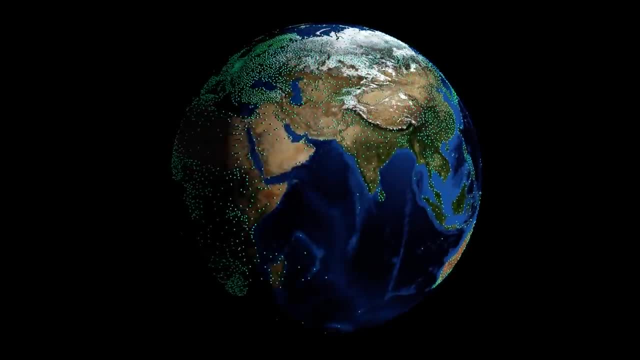 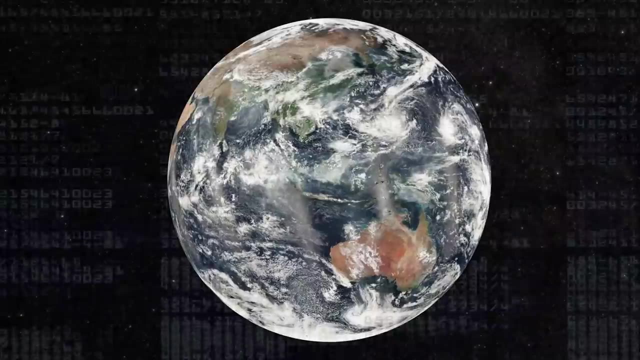 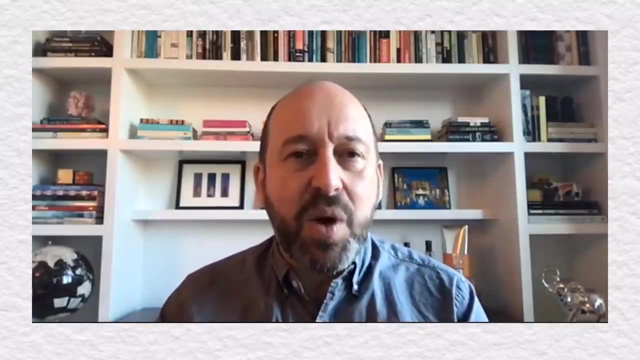 around the world. We use the information that's there to create a global picture of what's happening And that gives us a very accurate estimate of how any year ranks or what the what the anomaly is for any one year compared to what happened in the 19th century or what happened in the middle of the 20th century. 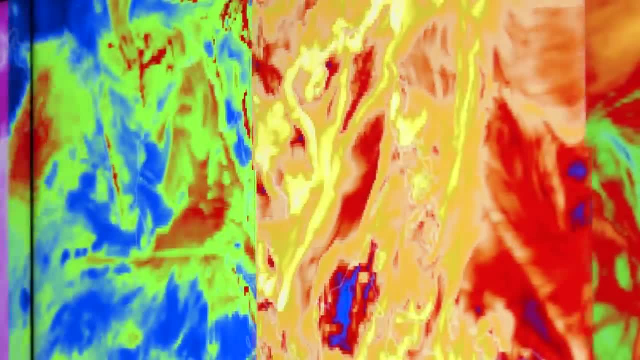 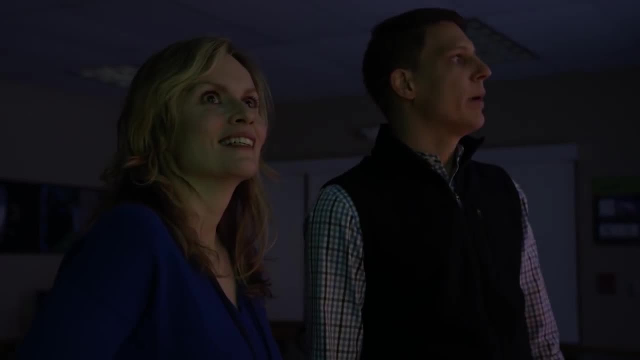 So we have our statistical reconstruction of Earth's recent climate. But in research science we like to check our work. There are a couple of ways we can do this. First of all, teamwork. Our colleagues at NOAA and at other agencies and universities around the world also create their own records. 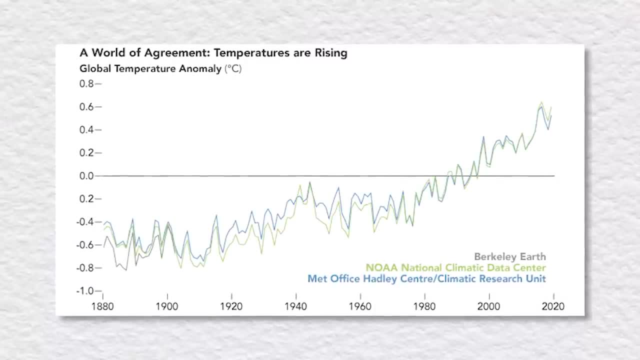 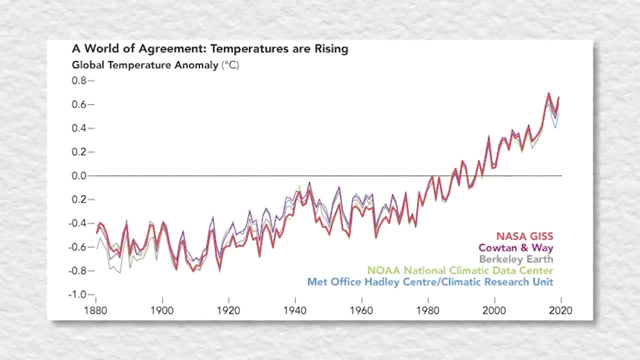 And we can line them up side by side and see just how closely they align. Everyone's independent climate records show the same thing: Earth is warming significantly and rapidly, And here at NASA we have an even cooler way to check our work: space. 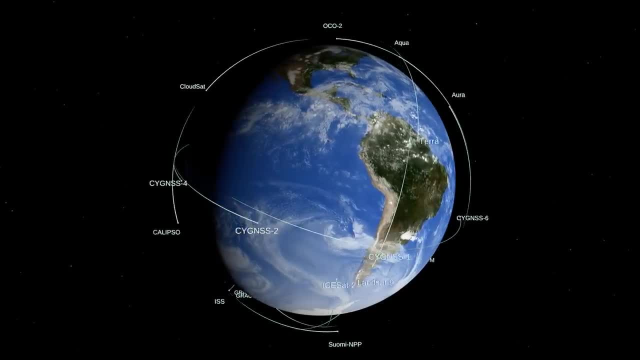 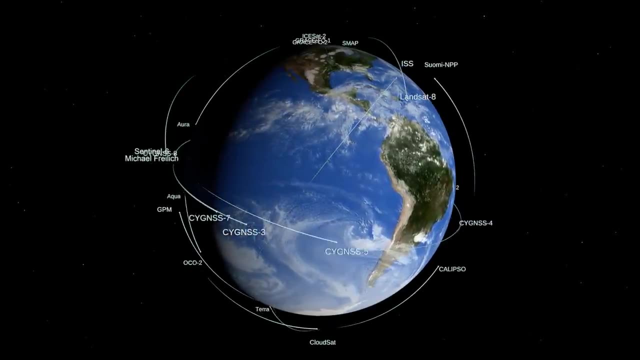 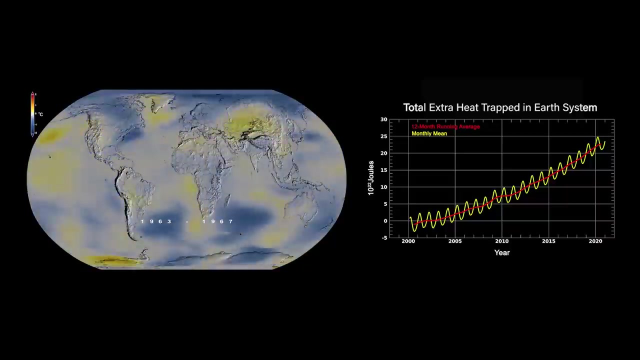 Right now we have more than two dozen satellites dedicated just to studying our planet. Satellites can take measurements of the entire planet and line them up with our estimate of global temperature change And, sure enough, they also match Our measurements from space, match up well with what our analysis tells us. 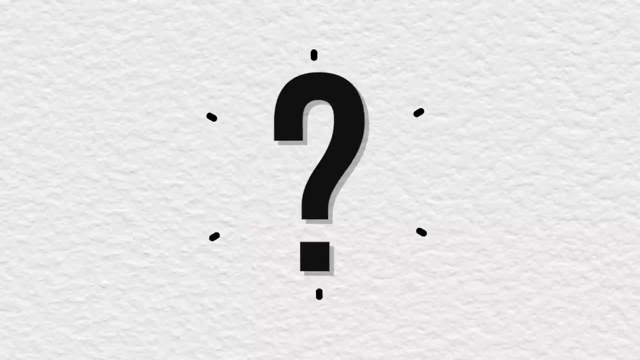 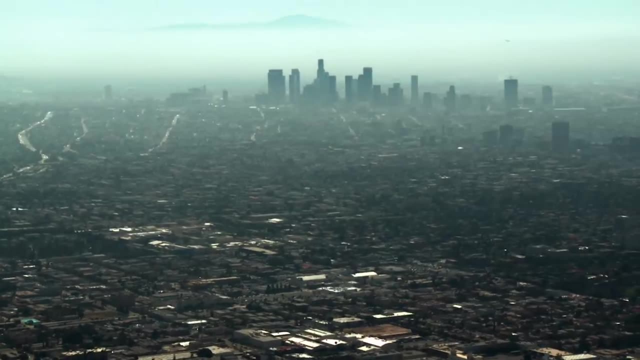 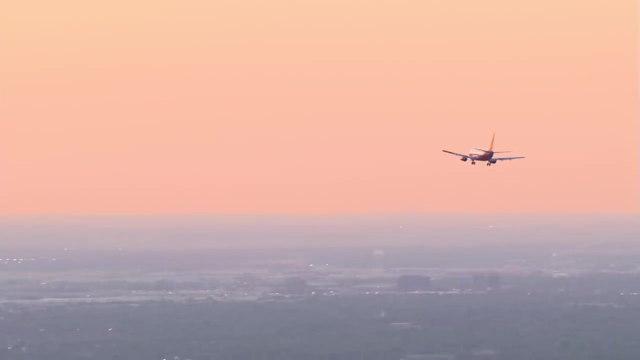 Earth's climate is warming. The next big question: Why is our planet warming? Well, let's jump back to the Industrial Revolution. The release of carbon, mostly carbon dioxide- The release of carbon, Carbon dioxide from human activities like driving cars, flying planes and industrial burning of fossil fuels is responsible for the majority of climate change. 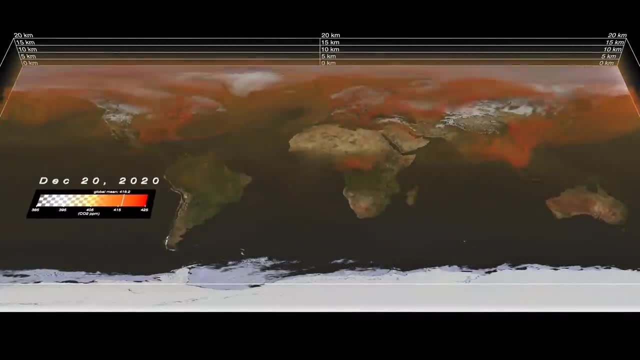 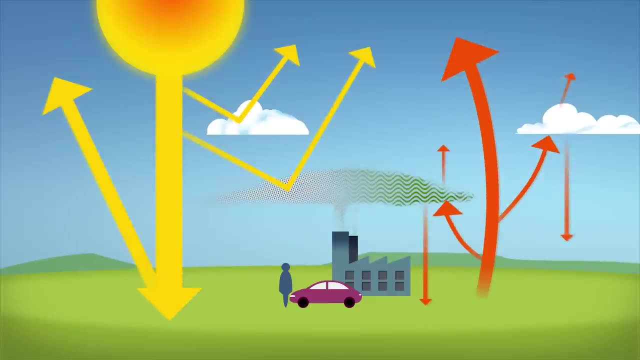 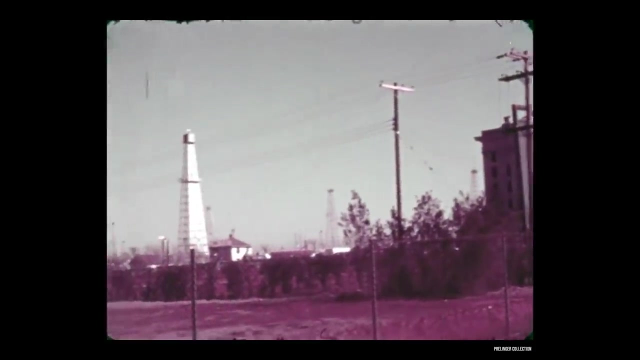 Carbon exists in stores underground as oil, gas and coal. When we burn it, we release it into our atmosphere, where it traps excess heat coming from the sun, raising the temperature. We've known for more than a century that carbon dioxide added to our atmosphere traps additional heat and is a major contributor to the greenhouse effect. 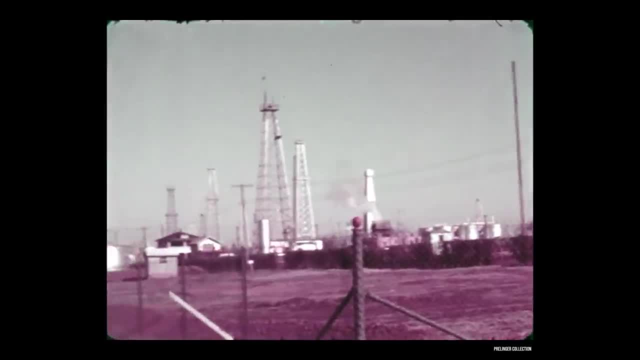 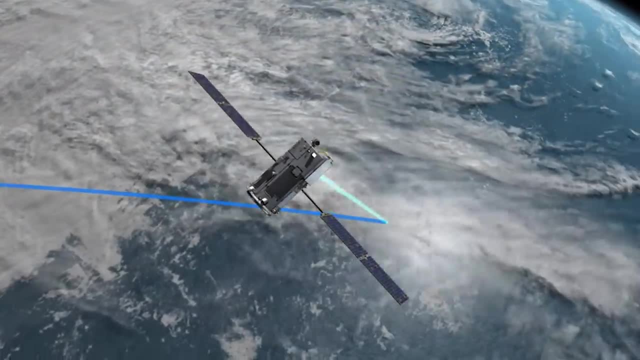 So we can also track the concentration of carbon dioxide in our atmosphere, the primary cause of the current climate change, Both from space, using NASA satellites like the orbiting Carbon Observatories 2 and 3, and from the ground. If you've heard of the Keeling curve, you're familiar with one of these records. 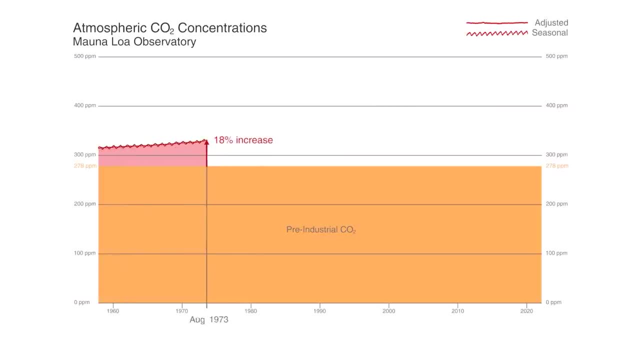 Researchers have been taking daily measurements of atmospheric carbon dioxide from Mauna Loa, Hawaii, since the 1950s. From space in the ground, the signal is clear: There's a lot more carbon in the atmosphere. It's heavier than there used to be. 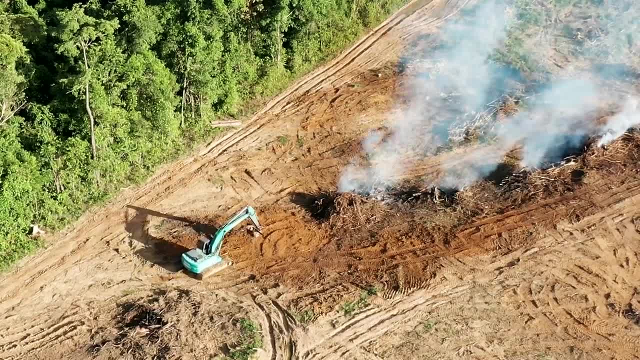 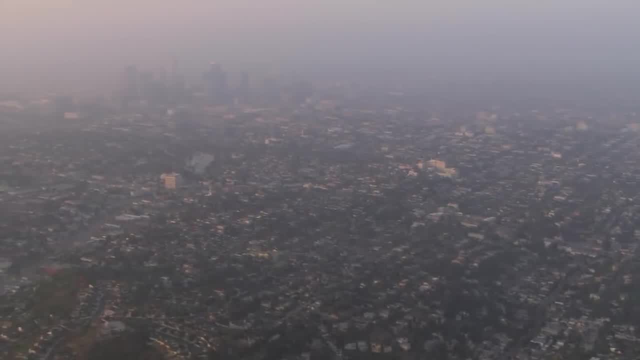 Other things have changed too. We've chopped down tropical forests, caused the ozone hole and filled the air with soot, smog and other kinds of air pollution, And this is on top of natural variations caused by the dynamics of the ocean or volcanoes, or variations in the sun's activity. 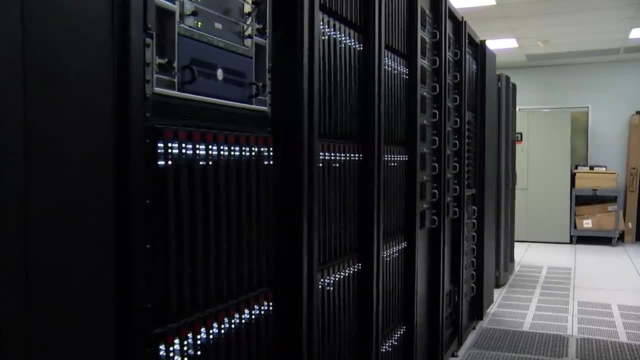 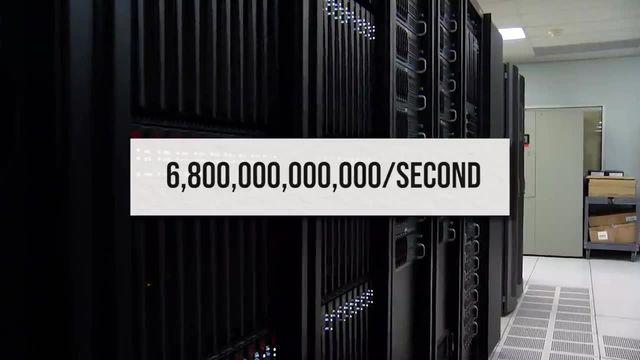 And so we can ask whether it's human activities warming our planet. At NASA, we have some big and powerful computers able to make 6.8 trillion calculations per second. We put these huge supercomputers to work to recreate Earth's climate. 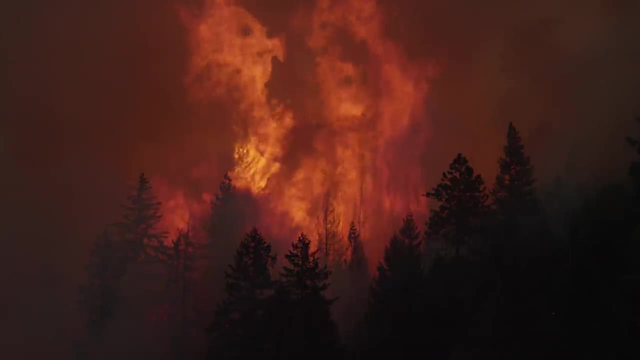 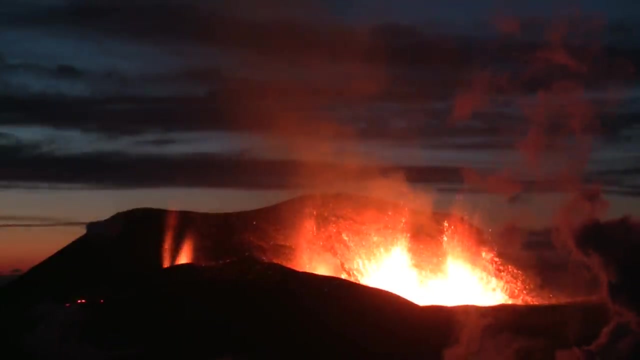 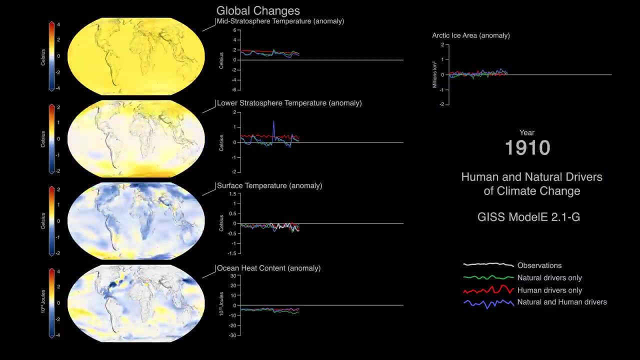 So we have thousands of ideas of what could naturally cause climate change. We have 4 billion years of history where nearly anything and everything you could imagine has impacted Earth's climate. But each of these events has their own distinct fingerprint which we can identify: a pattern of behavior with natural variability. 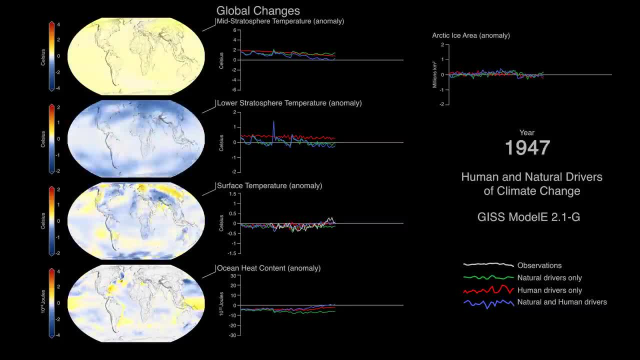 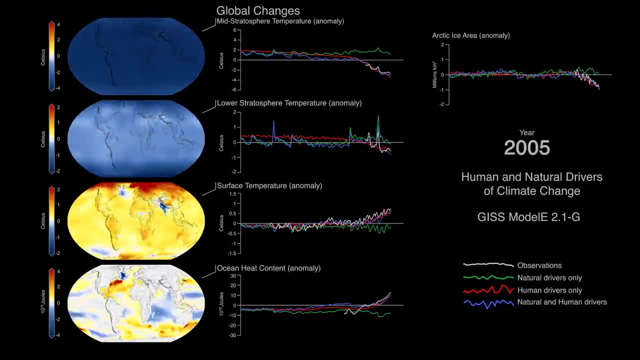 Using supercomputers, we can run simulations of natural climate, drivers, solar energy changes, wobbles in Earth's orbits, ocean turnover, volcanic eruptions, and we can run simulations of human effects. And what we've seen is It's us. 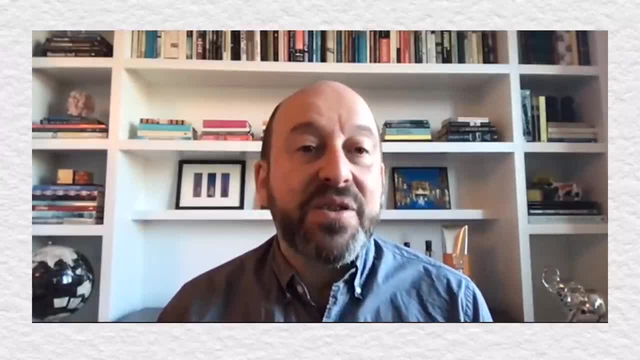 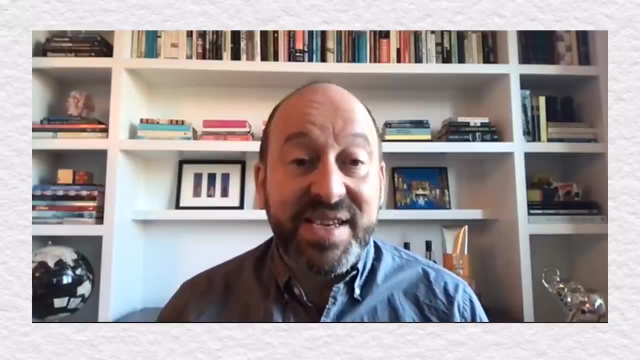 There's no way around it. Looking at the evidence, we're the force that's enacting these changes. I am so proud of our ability to understand the climate, but I'm terrified of what we've found. But it's not just the causes of climate change. 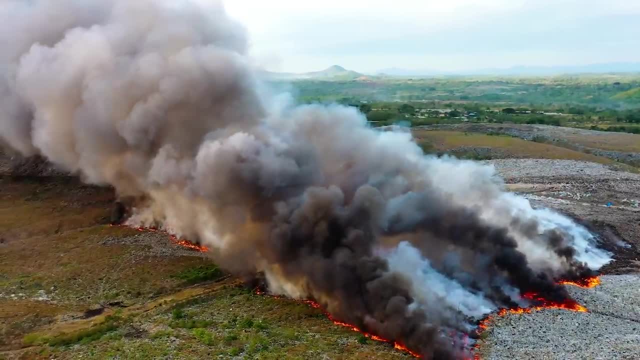 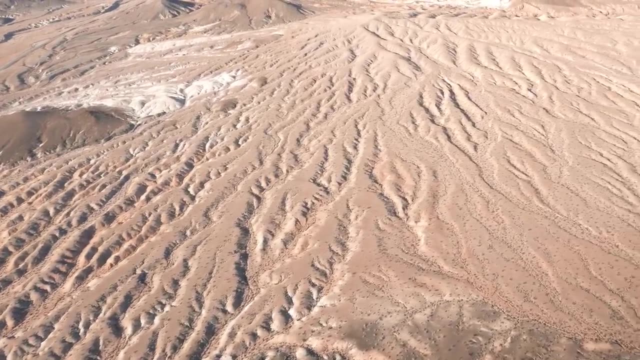 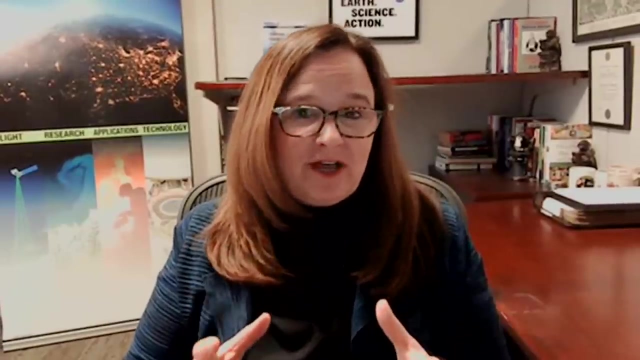 It's also the effects, Because it's not just about knowing why our planet is warming, It's also about understanding and preparing for the effects of added warmth. Measurement of global average temperatures is so important because it's one of the most direct indicators of Earth's changing climate. 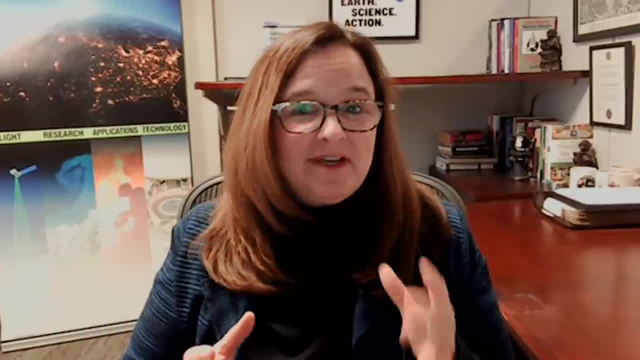 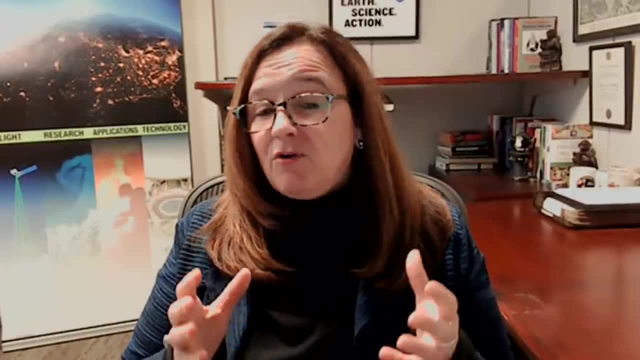 But the Earth is really a system of environmental systems- Land, ocean, atmosphere and ice- And changes in one system impact the others. Our oceans are our first line of defense in climate change because they absorb so much of the extra trapped air.